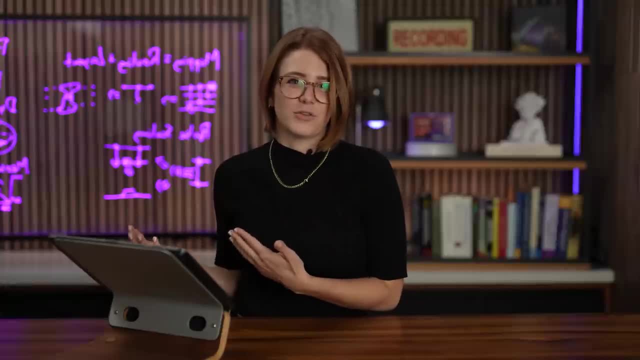 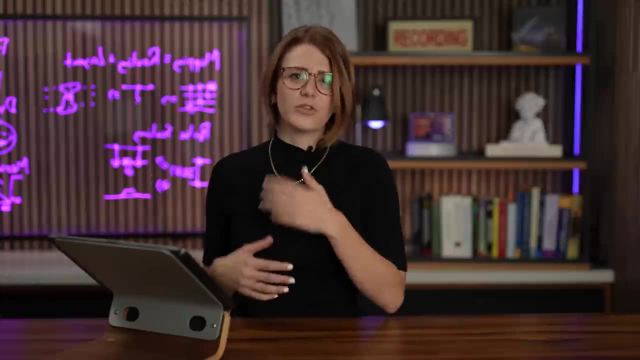 for instance, we always say: if a tree falls in the forest and no one is around to hear it, does it make a noise? If the answer is yes, this would be an example of definite realism. realism. So he assumed only those two things in his mathematical derivation And he was 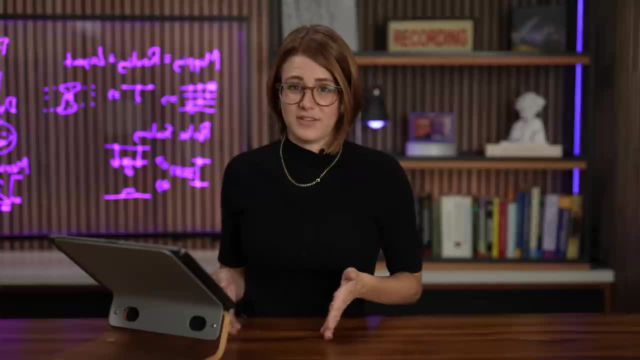 able to show that there are certain qualities, quantities that you can measure, that are bounded by classical physics, if you assume only local realism. And essentially he was able to show, on paper at least, that quantum mechanics was incompatible with any classical theory. So anything that was basically including local realism could not possibly work with. 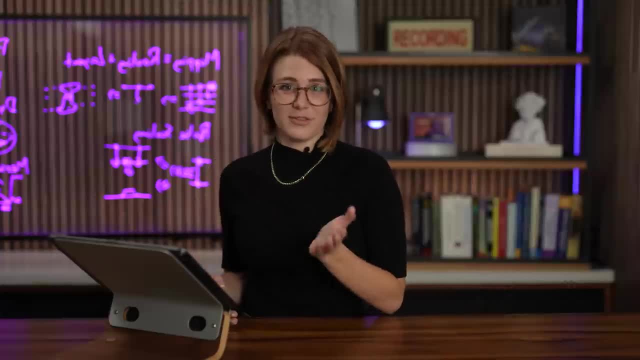 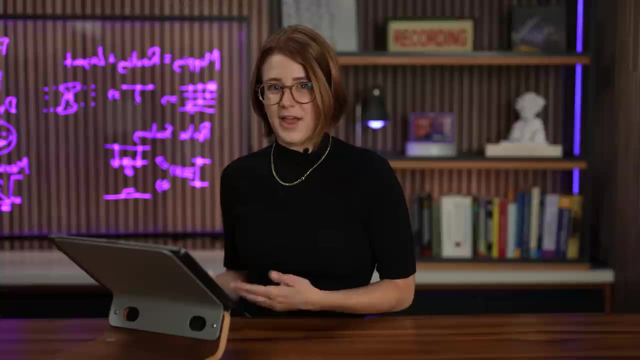 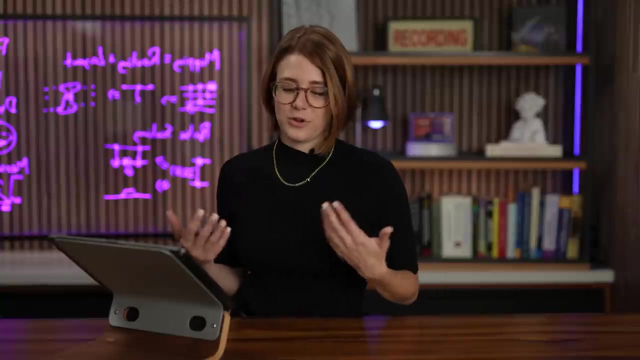 quantum mechanics. So now, a few years later, John Clouser came along and he was reading Bell's theorem And he thought that this should be something that was able to be done experimentally. So he was able to actually perform an example in the laboratory for the first time. I even 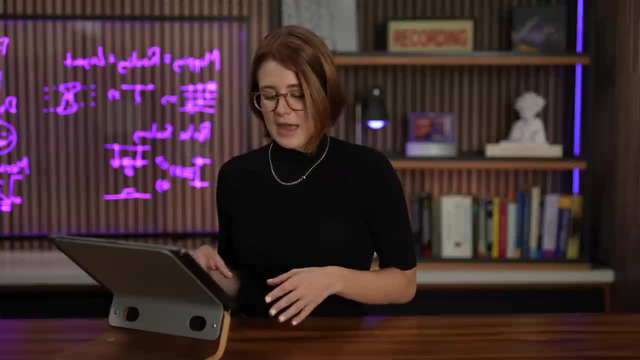 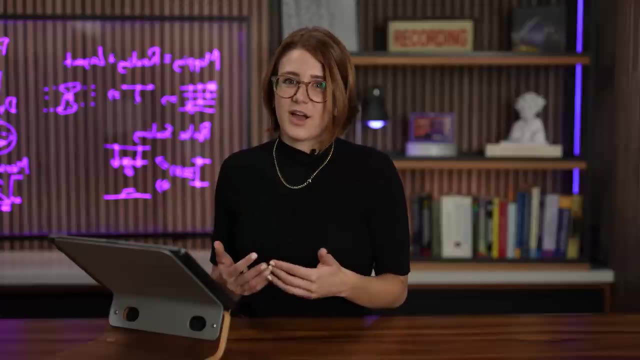 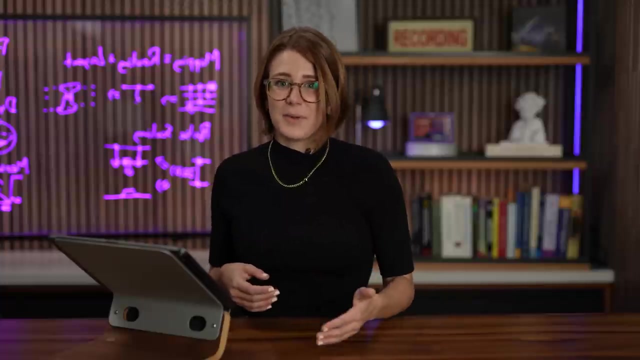 wrote a paper on this, And it showed that, indeed, nature behaves as weirdly as predicted, And so, in essence, Einstein was wrong in his EPR paper, And this led to groundbreaking work later on from Alain Aspect, who was able to perform even more tests of Bell's inequality. 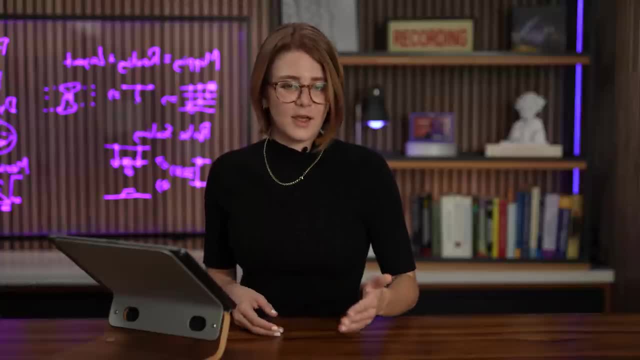 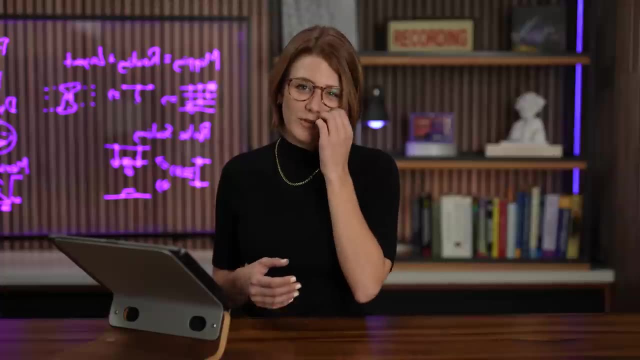 and close some of the loopholes, so to speak. And then this led to Anton Zellinger, who was able to show the demonstration for the first time, And this led to the first time of quantum teleportation, which is not what you might. 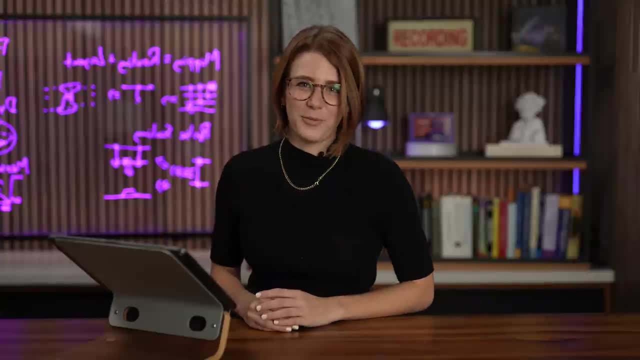 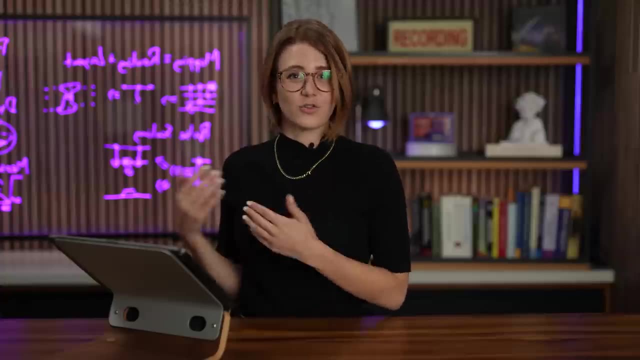 think It's not at all like Star Trek. People are not teleporting across the room, But instead quantum teleportation is a way to entangle or correlate quantum particles in such a way that you can transfer quantum information from one to another. 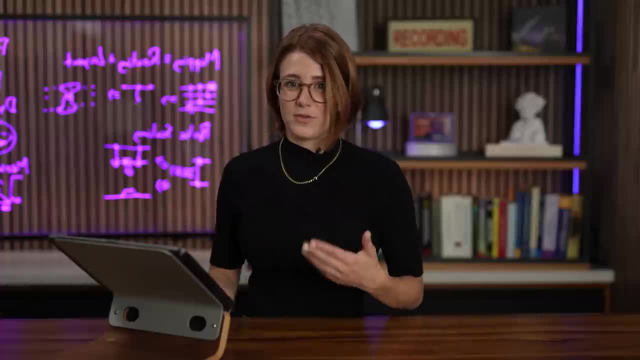 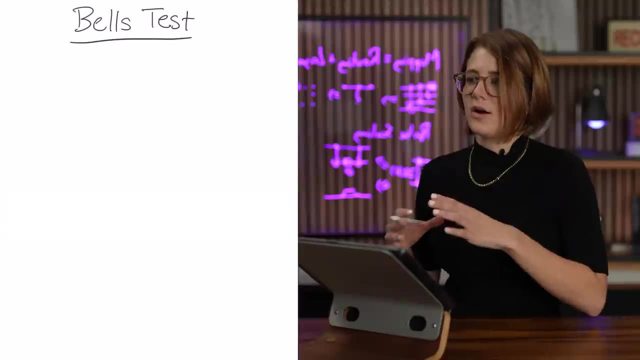 So, in order to really understand why this is so important and why this is so groundbreaking, I want to go back and look at a very specific demonstration of Bell's tests for you. There are, in fact, many different examples, bell-type theorems- that can be shown, but we're going to look at really one. 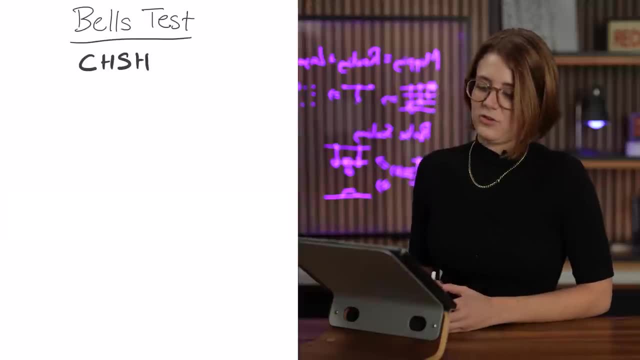 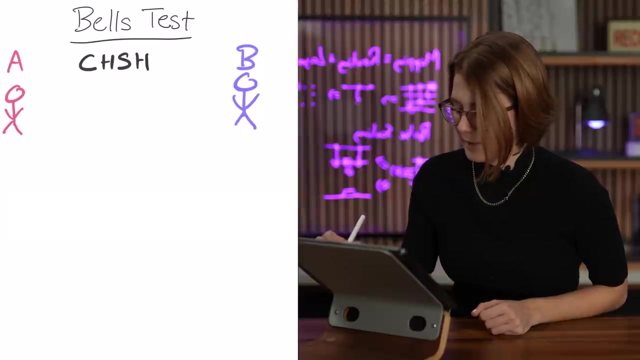 specific one today, which is called the CHSH test or the CHSH inequality, And so what you need to do for this thought experiment is first imagine a person named Alice and a gentleman named Bob, and they are standing some distance, far away from one another, And then there's another guy in the middle. let's just 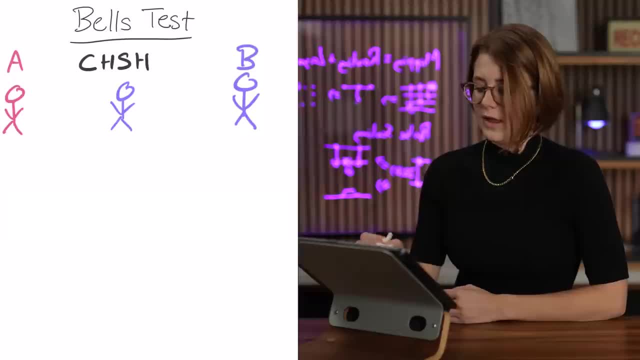 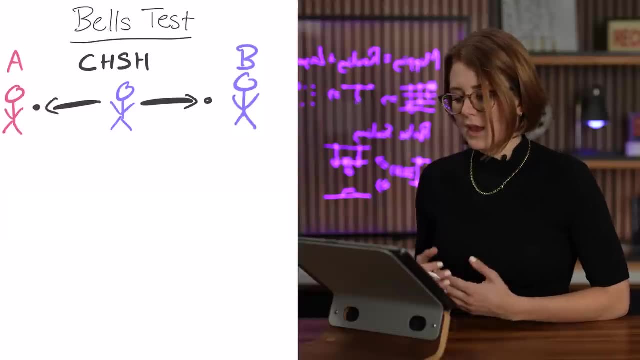 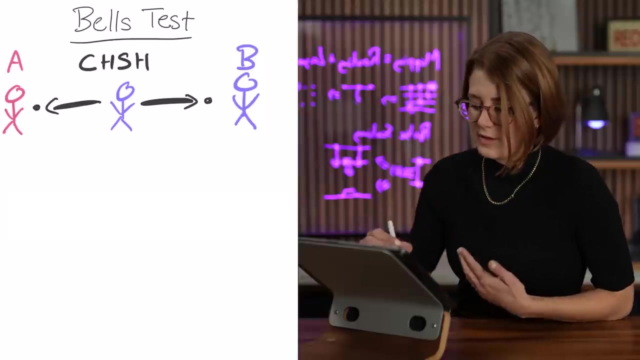 call him Victor, and he's going to send a particle to Alice and to Bob at the same time, And Alice and Bob are going to perform, every single time this happens, one of two measurements. They're going to either measure the x-projection or the. 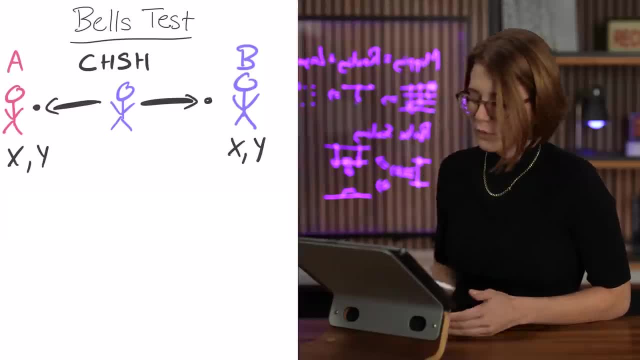 y-projection of this particle, And so you can only measure one at a time. So in order to have a good understanding of the measurements of both, they have to perform this experiment multiple times, And it's important to note that every time Alice receives a particle, Bob also receives a. 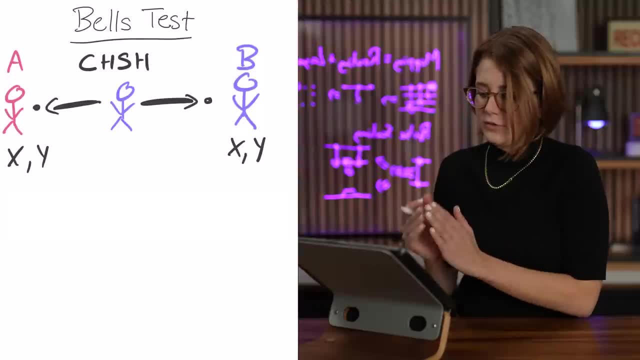 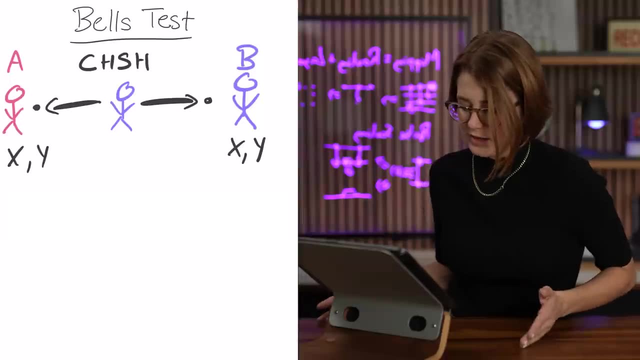 particle And again, the only thing we're really assuming here is local realism. So these particles are not moving faster than the speed of light. Bob and Alice can't call each other faster than the speed of light and communicate information, nothing like that. And these particles also have these definite 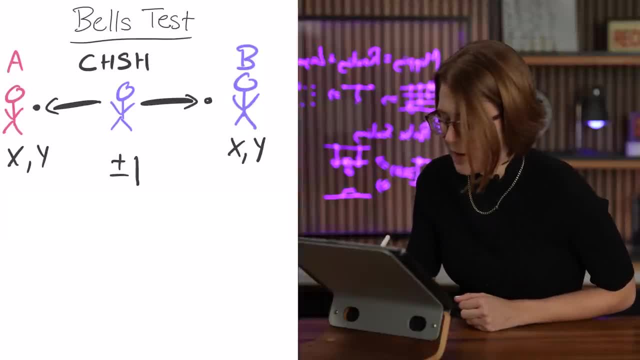 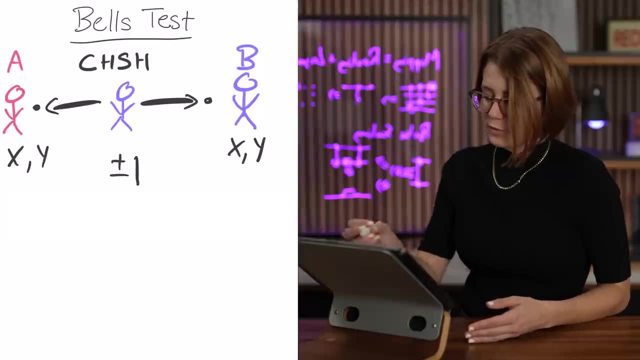 values that are either going to be one or minus one, because let's just say they're normalized. So the values for x and y for Alice and x and y for Bob can only be one or minus one. They are binary. So now, at this point, we need to write down what is known as the 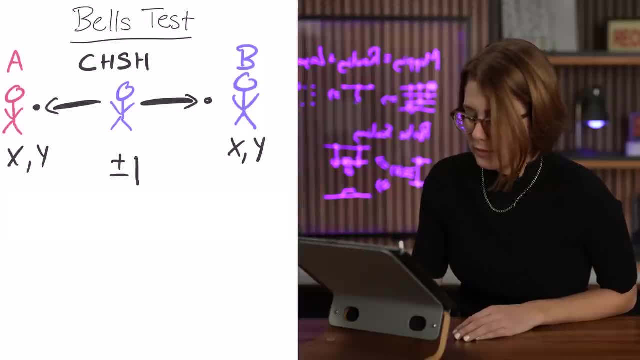 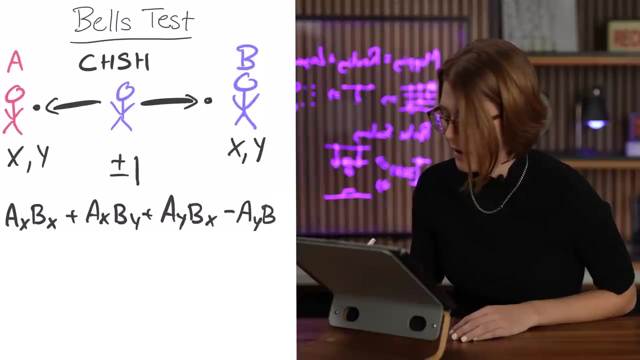 CHSH value. So this is like: so: Alice's measurement of x times Bob's measurement of x, plus Alice's measurement of x, Bob's measurement of y, Alice's measurement of y, Bob's measurement of x, and then you subtract from that sum Alice's measurement of y and. 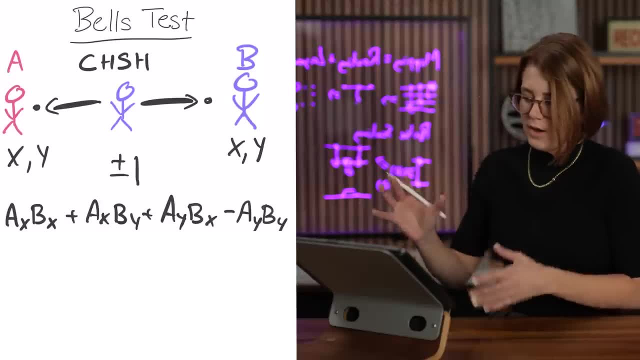 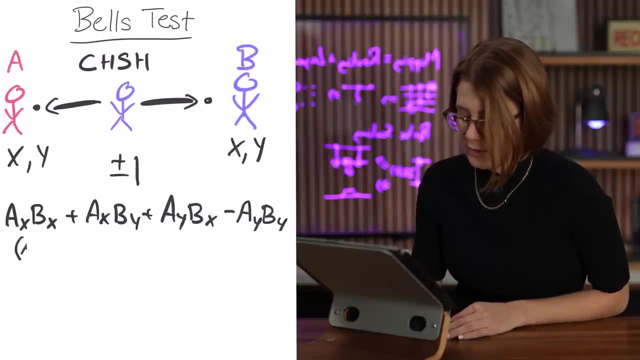 Bob's measurement of y, And it really doesn't matter where this quantity comes from. The fact is, if we look at it a little bit closer, we can factor out the Alice quantities from the Bob quantities and you see, we would get something. 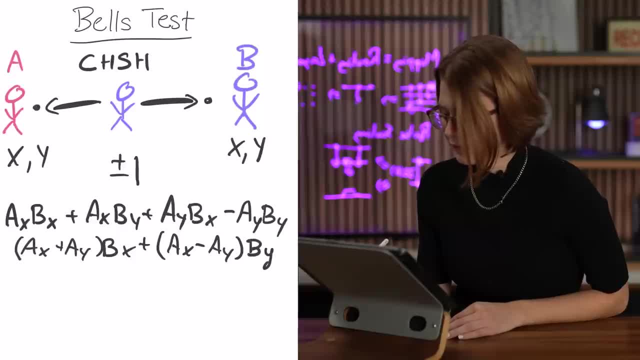 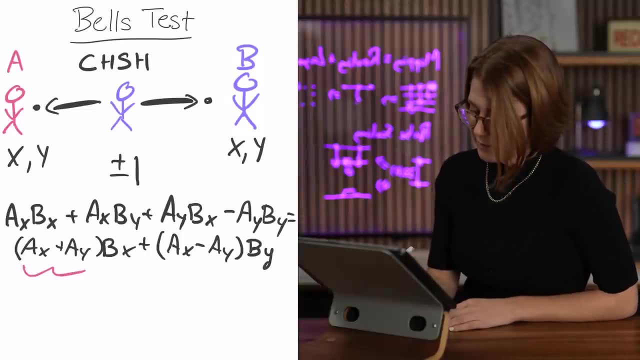 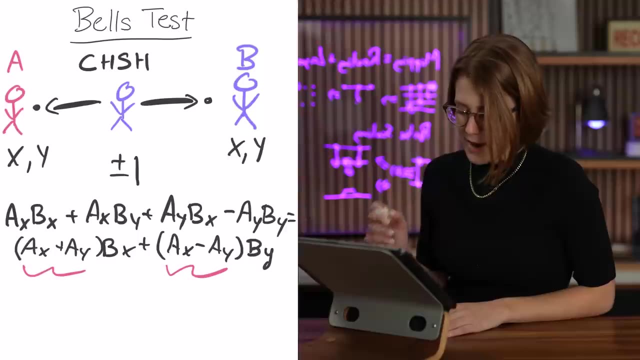 like this, And I drew this for you here: a little equal sign there at the end. So you can see that either this value every time the experiment is performed, or this value is going to be equal to zero, because either you are measuring one minus one or you're going to have minus. 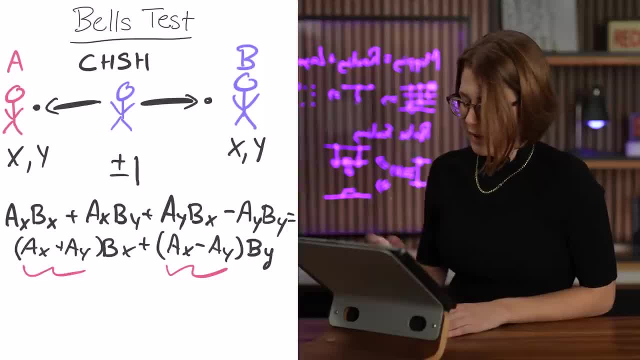 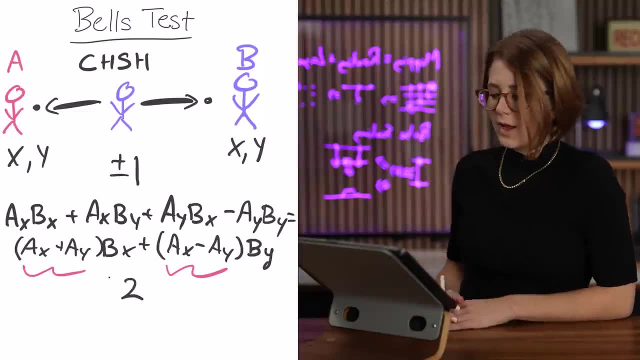 one plus one. The values again can only be one or minus one, So the maximum value this quantity could take on is equal to two At most. But remember, we're running this experiment many, many times, So say we ran. 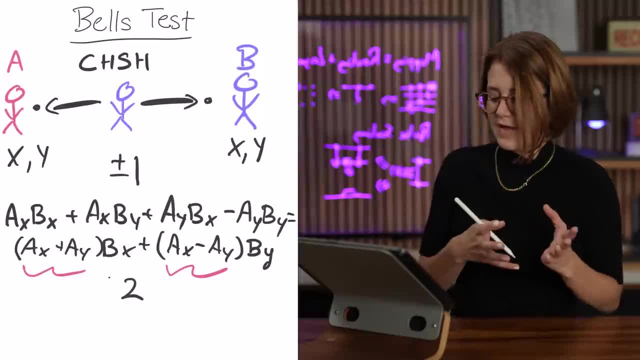 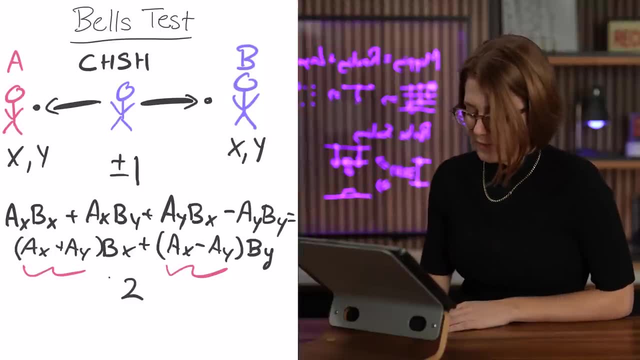 this experiment hundreds of times and we're measuring a few different values every time. Alice is measuring x and y, and a few different values every time Bob is measuring x and y. That means that this is actually bounded by two again, but it can be equal. 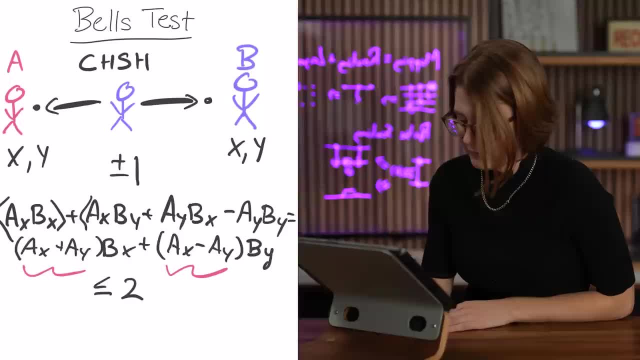 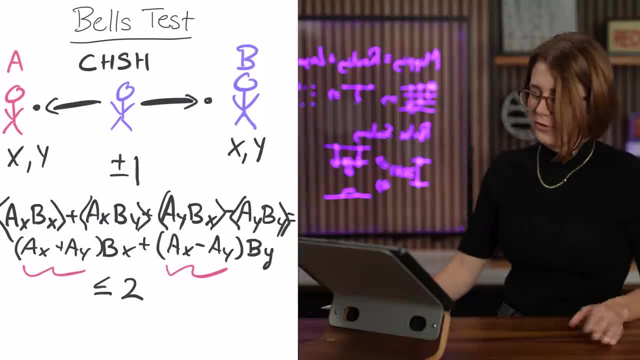 to two or less than two. once we take the averages- And that's what these little brackets mean here- We're going to take the average of two, and then we're going to take the average of two of all of these measurements. all right, so this value has to be less than two if the only 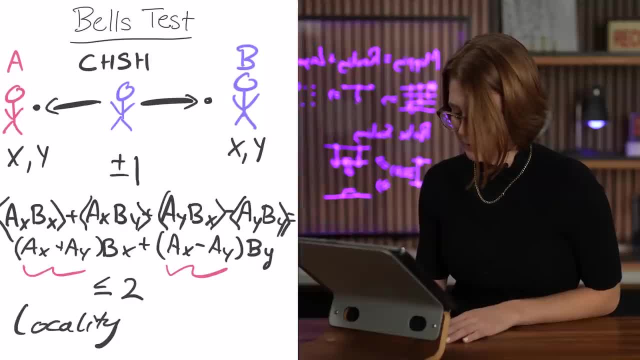 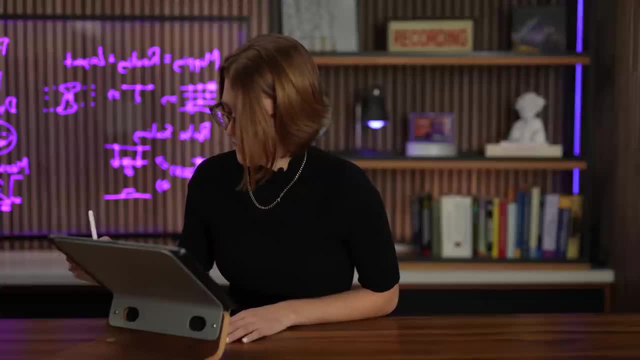 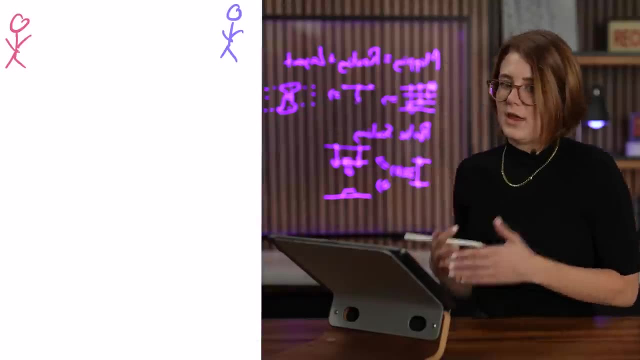 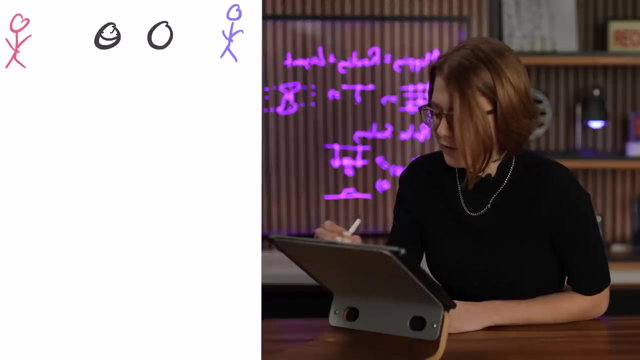 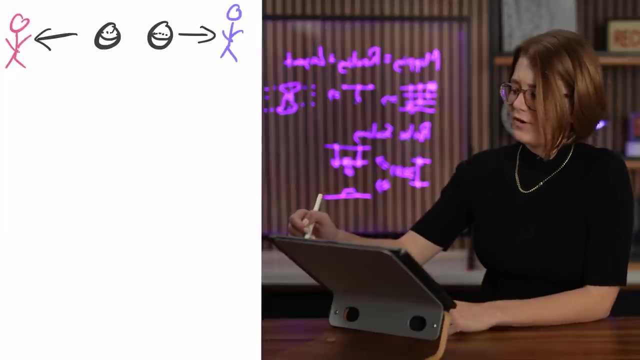 assumptions we are making are locality and realism. however, let's think about this experiment again slightly differently. let's now assume that, instead of a particle, just a random object allison bob are receiving. they are going to be receiving entangled cubits. these are cubits. it doesn't matter how they were entangled originally at the beginning. let's just say: 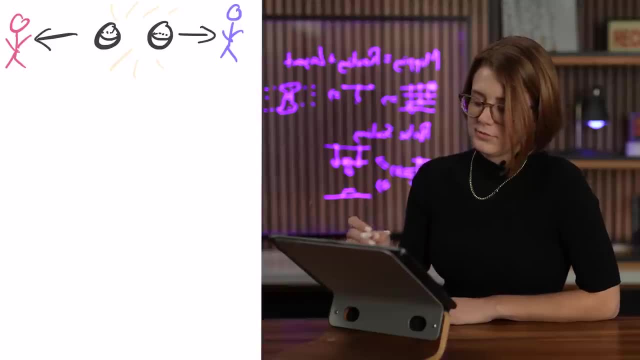 that they are. what you're actually going to measure, once you perform this experiment hundreds of times, is that this quantity is going to be approximately 2.8, not two, not less than two. we know for sure that 2.8 is greater than two. which means that if these qubits obey the laws of quantum mechanics, which we know they do, quantum mechanics violates Bell's inequality. It is incompatible with local realism. So either something is moving faster than the speed of light or these particles do not have definite values. 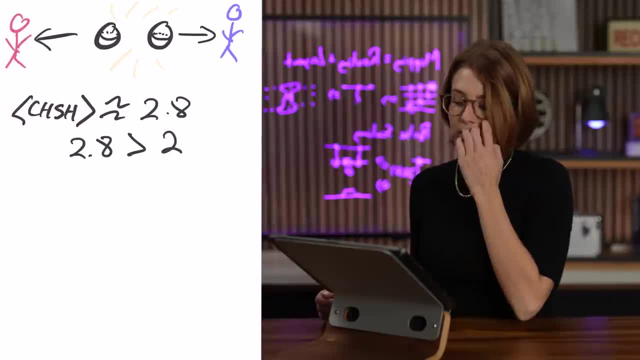 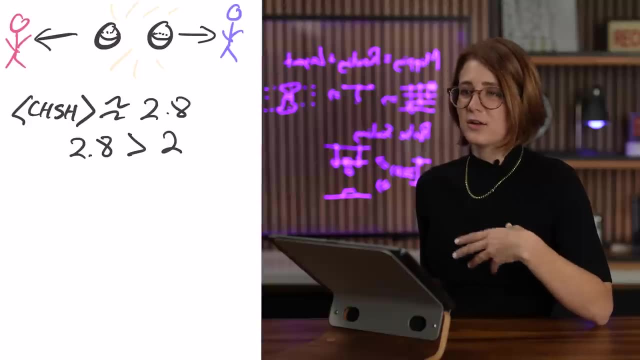 before they are measured, And now a lot of people, I think, misconstrue what this actually means. Some people think that this opens the gateway for faster-than-light communication. This is not the case. Let me be very clear about that. 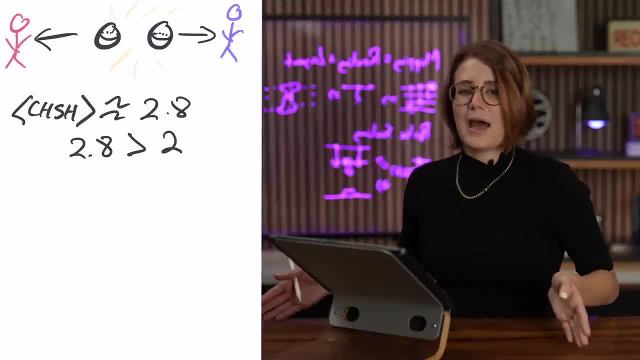 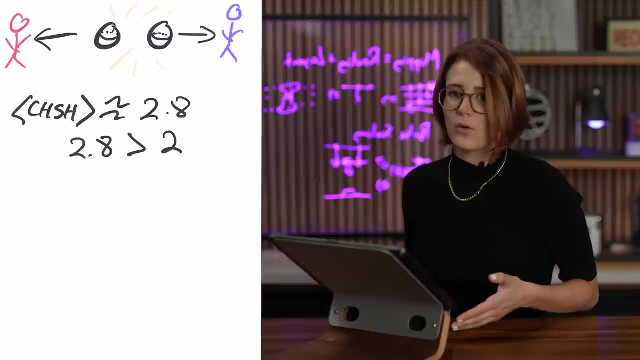 because this is a really easy mistake to make. Bob and Alice are not communicating with each other faster than the speed of light. There's no possible way to do that. The particles become entangled and when you measure them, say Alice measures one. 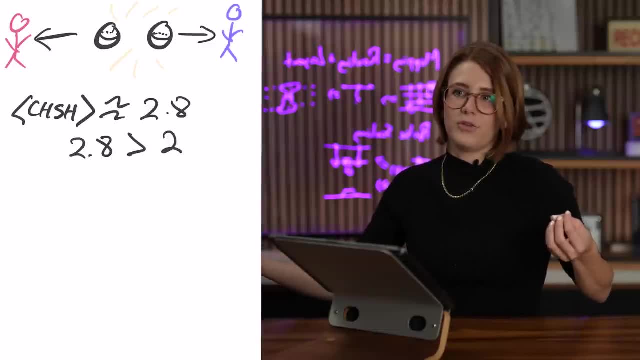 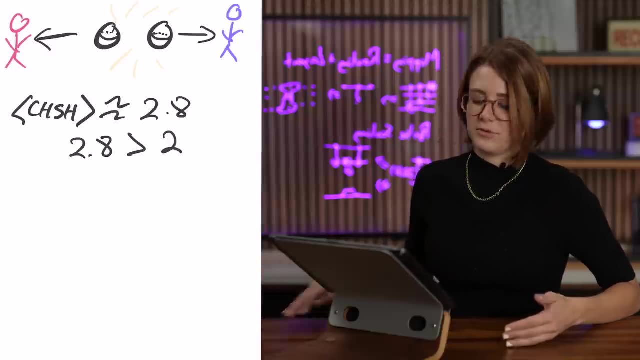 we know that instantaneously, the other particles are going to be going to choose the opposite correlated value- negative one. But that does not mean that Alice and Bob are able to communicate with each other faster than the speed of light. No information is being transferred at that speed. 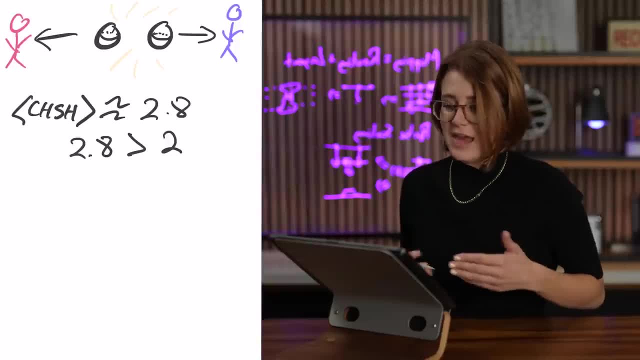 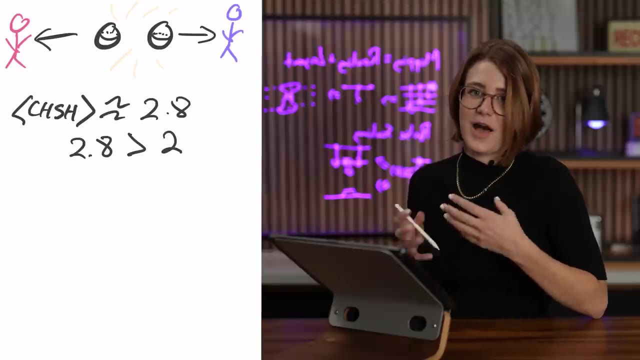 So that's really important to know. And since there's no evidence of anything in the universe traveling faster than the speed of light, the way that most scientists have interpreted this is that we have to give up the idea of realism. These quantum particles actually do not have. 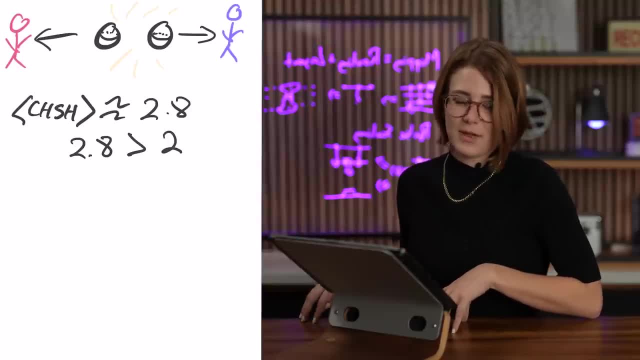 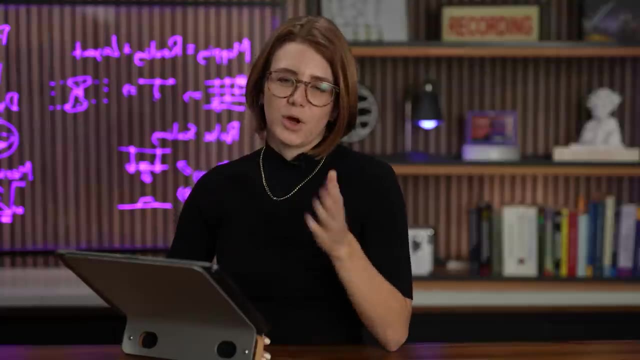 values that are specific to them before you measure them. They are instead described by what Einstein called and resented the wave function, And so it has some probability of being in either state one or minus one before you measure it. And you might be wondering: where does this 2.8 number come from? 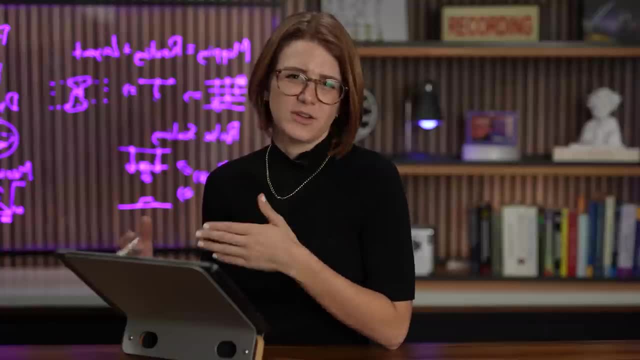 Certainly it's greater than two, and we can understand that it does indeed violate this inequality, But where does this 2.8 come from? And so, if you're interested, I'm going to give you a couple of examples. So, if you're interested, I challenge. 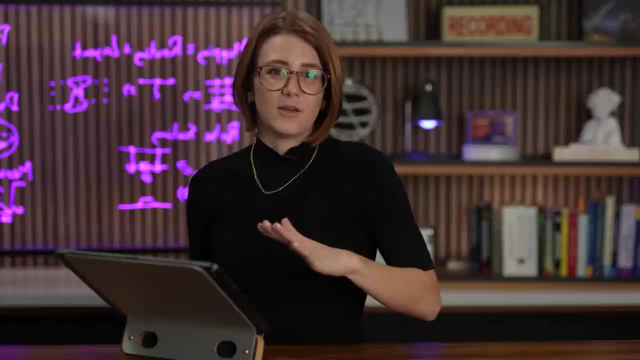 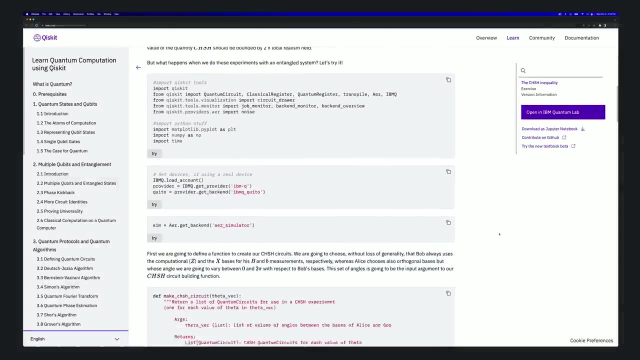 you to go online to the Qiskit textbook- and the link is linked below in the bio- and to try your hand at this experiment for yourself. right now There is a tutorial actually already published online on the Qiskit textbook on the CHSH inequality. 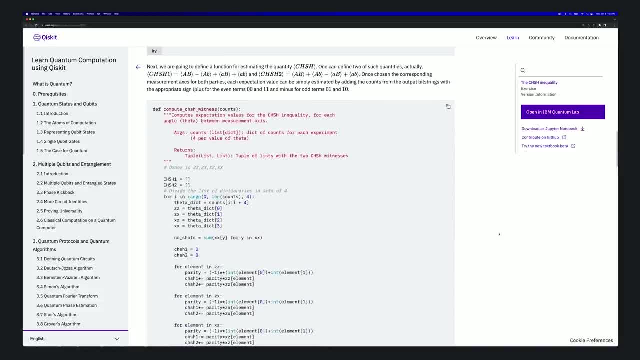 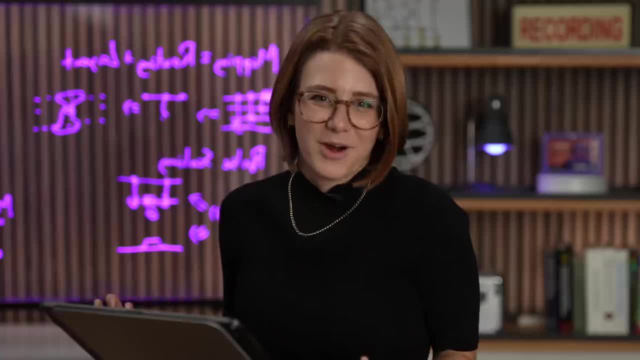 And you can run the experiment from your couch or wherever you are right now and see, indeed, that you are going to get a number that is approximately 2.8.. And while you might not win a Nobel Prize for doing this, because lots of experiments in this vein- 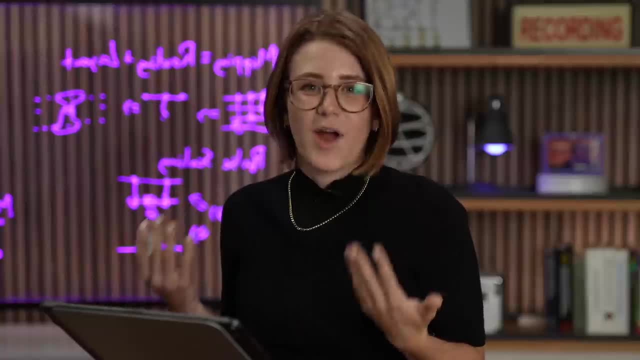 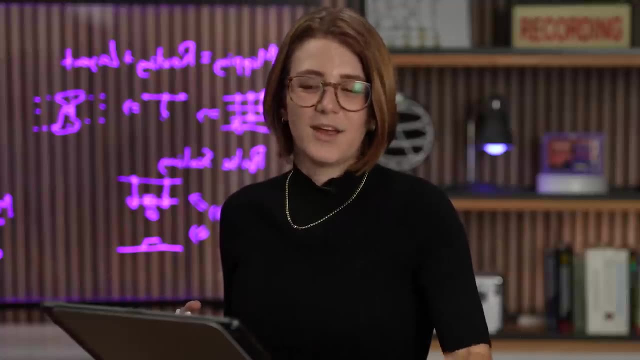 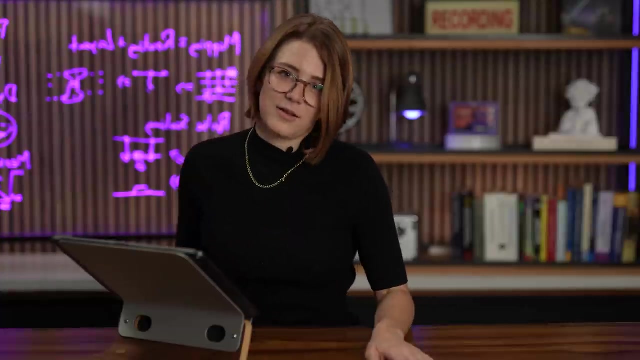 have been done at this point. I still think it's miraculous that we have gone in a few decades from an experiment that is Nobel Prize winning to an experiment that you can do- that I can do- from anywhere in the world. So what this showed is that quantum mechanics is even